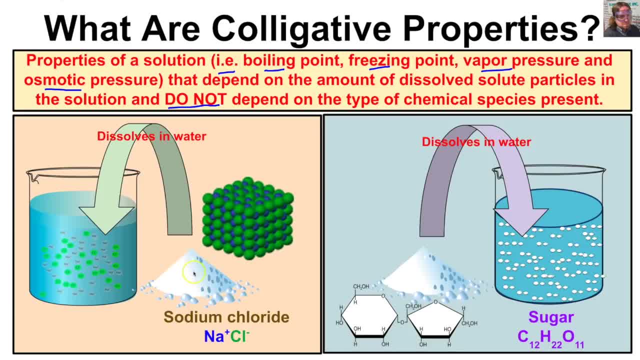 for example, if we take a look over here here we have a mound of sodium chloride or table salt, And if we take a look at what table salt might look like on a microscopic level, it looks like we see right here. It forms this crystal structure that we see right here, And so if we take a look, we have a bunch of 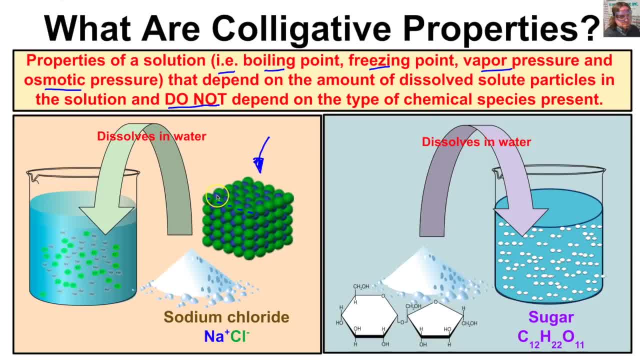 chloride ions, which are negative, tightly packed in with some sodium ions, which has a positive charge, And we learned that in an earlier video. when you put this in water here, it's going to dissociate. It's going to dissolve and dissociate, It's going to break apart into chloride ions that 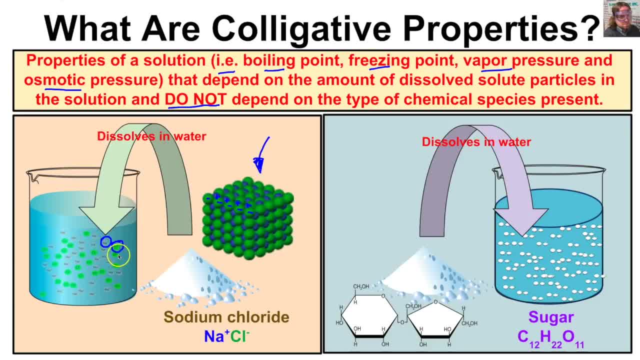 are floating around in this water and sodium ions that are floating around in this water. So what ends up happening is that any time you have particles like this that are floating around in water, it's going to increase the boiling point of that solution and it's going to decrease the freezing point of that solution. So when we add 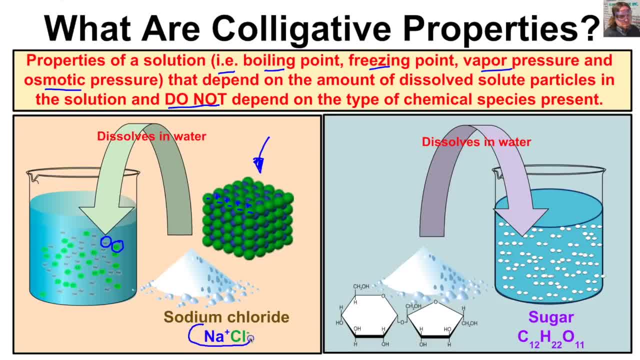 an ionic compound like salt or sodium chloride to water. it's going to dissociate and produce some ions that are free floating in this water right here, And that's going to cause it to have its boiling point increased and its freezing point decreased, And the same thing with sugar. 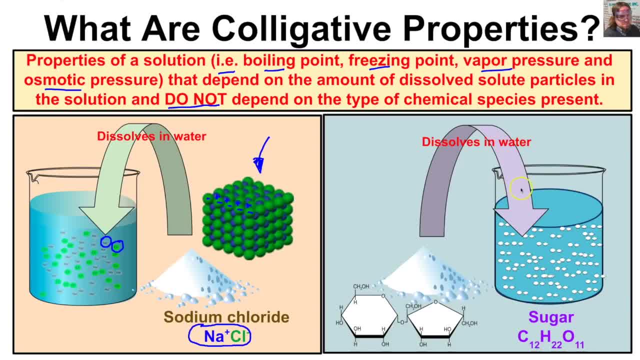 If we take some sugar here and we put sugar in water, we know from prior experience that it too is going to dissolve, right. And so we can take a look right here and yes, sugar is going to dissolve, but it's not going to dissociate, It's not going to break apart like we see this ionic 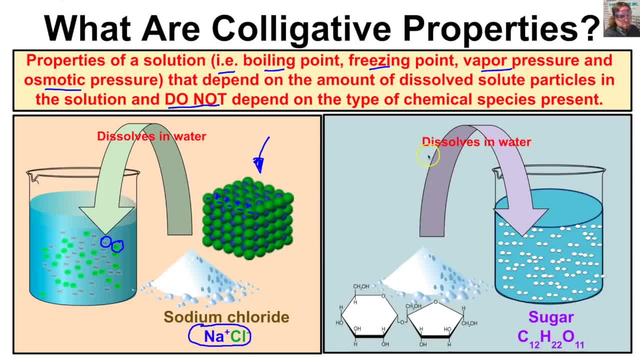 compound do on the left-hand side. And so, if we take a look right here, this sugar is going to dissolve in water, And so its freezing point, the freezing point of this solution, is going to decrease, and the boiling point of this solution is going to decrease. And so, if we take a look right, 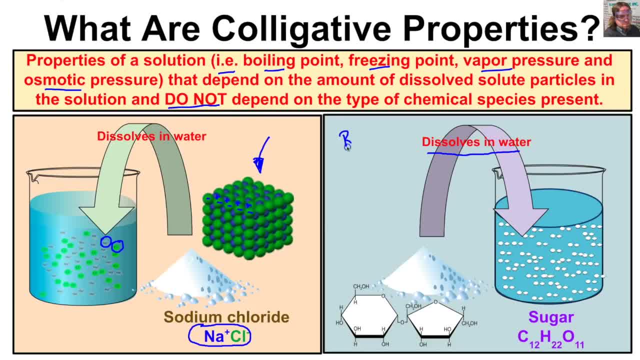 here the boiling point of this solution is going to increase as well. So in both scenarios- here the boiling point of the solution is going to increase. The freezing point of the solution here is going to decrease, And same right here, the boiling point of this solution is going to. 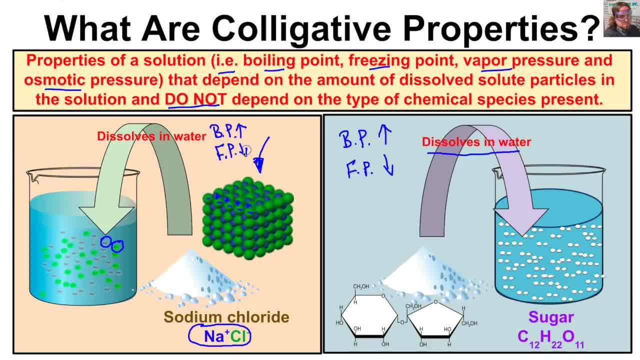 increase and the freezing point is going to decrease. But if I were to ask you which one of these will have a higher boiling point now and a lower freezing point, which one would it be, and why? Well, that's what we're going to talk about in this video. If we take a look over here, 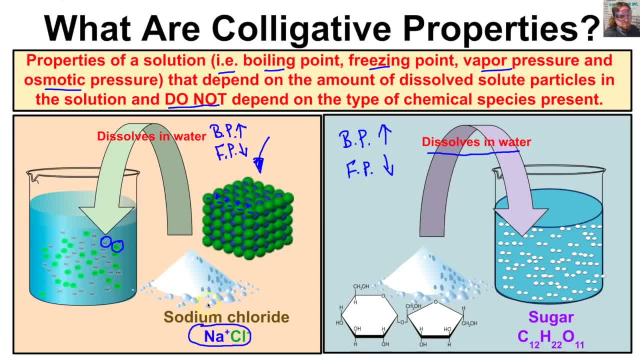 when we put sodium chloride in water, it's going to dissociate. And so if we have one mole of sodium chloride, it's going to produce two moles of particles. It's going to produce one mole of sodium ions and one mole of chloride ions, for a total of two moles. And so, because 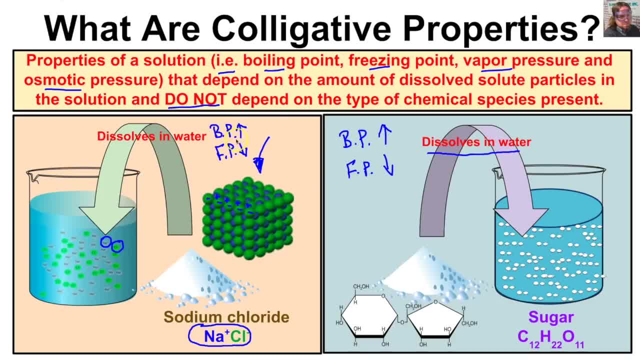 there's more dissolved particles in this solution. here the boiling point elevation is going to be greater and the freezing point depression, is going to be greater. If we compare this to just sugar, if we take a look at sugar, if I have one mole of sugar, it's not going to dissociate. 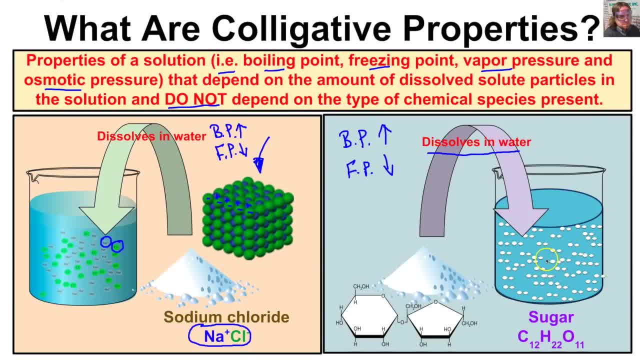 so it's going to produce, or there's only going to be, one mole of sugar particles that are floating around in this beaker of water here. So that is why sodium chloride dissolved in water is going to give a higher boiling point and a lower freezing point compared to sugar dissolved in. 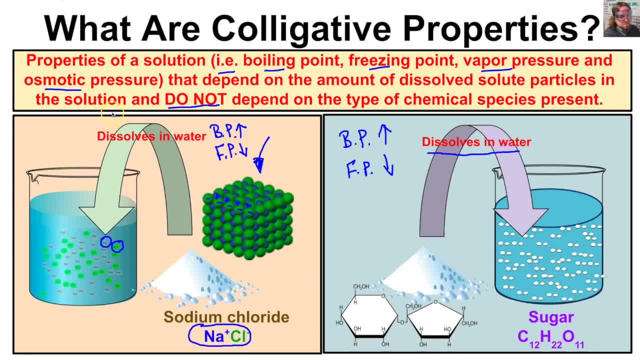 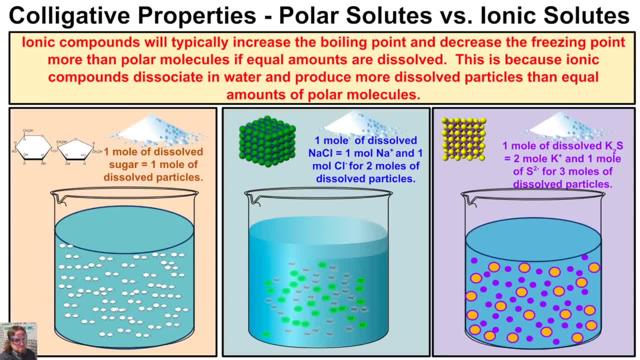 water. So let's take a look at a couple more examples of this phenomenon and compare and contrast the differences between them. And so it says right here that ionic compounds will typically increase the boiling point of sodium chloride. And so if we take a look at the 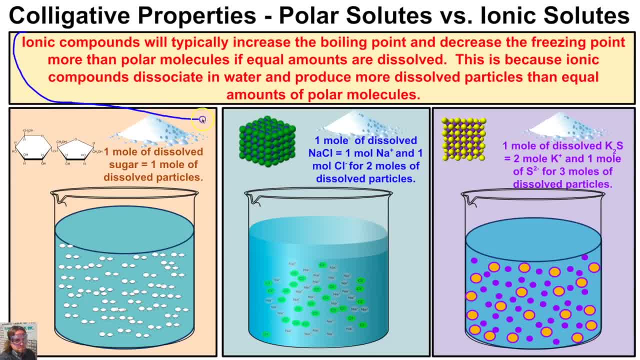 boiling point and decrease the freezing point more than polar molecules if equal amounts are dissolved. this is because ionic compounds dissociate in water and produce more dissolved particles than equal amounts of polar molecules. So right here, once again we have some sugar. 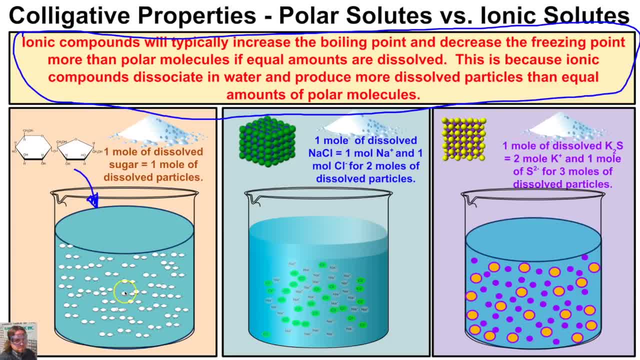 And when we put one mole of sugar in here, it's going to produce one mole of dissolved particles in this solution because it does not dissociate, It does not break apart. If we take a look right here, if we take this one mole of sodium chloride and we put it in here, 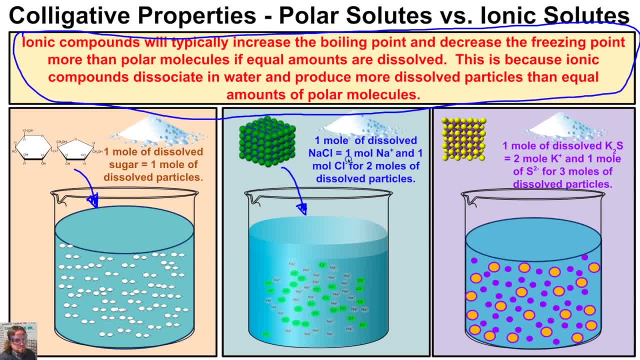 it's going to dissociate and produce one mole of sodium ions and one mole of chloride ions, for a total of two moles of dissolved particles. And if we take a look at this substance here, K2S or potassium sulfide. if we dissolve one mole of this in this solution right here or in this beaker of 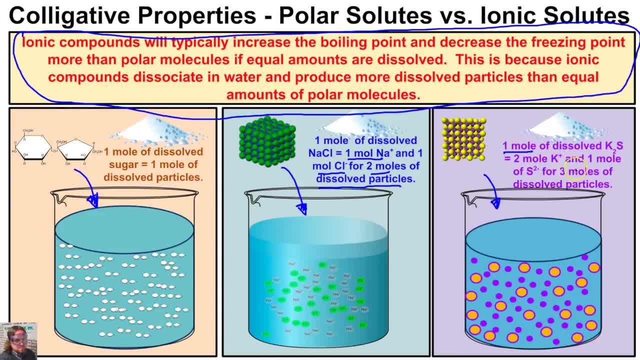 water right here. it's going to dissociate too, because it's an ionic compound, and it's going to end up producing one mole of sulfide ions and two moles of potassium ions, for a total of three moles of dissolved particles that are floating around in this solution. So if we asked which of these three solutes will cause a 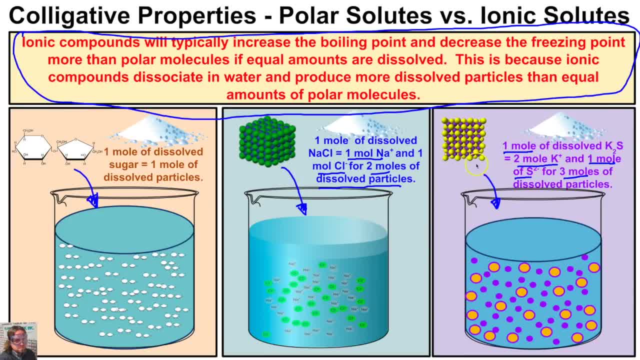 higher boiling point elevation and a lower freezing point depression. it's going to be this one right here. It's going to be this one right here because there's going to be three moles of dissolved particles in here, only two moles of dissolved particles in here, and only 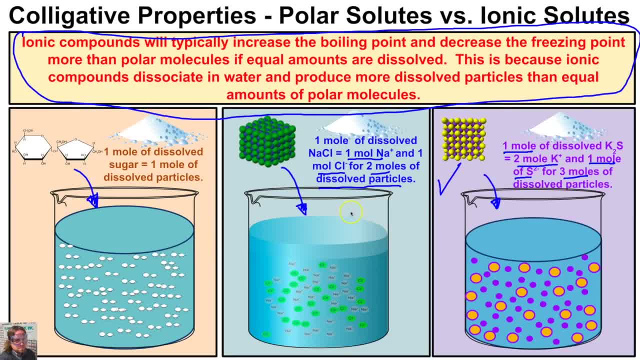 one mole of dissolved particles in here. So what we can do is we can actually use a formula to calculate the boiling point elevation and freezing point depressions of different aqueous solutions that have different types of solutes dissolved in them. So let's take a look at that right now. 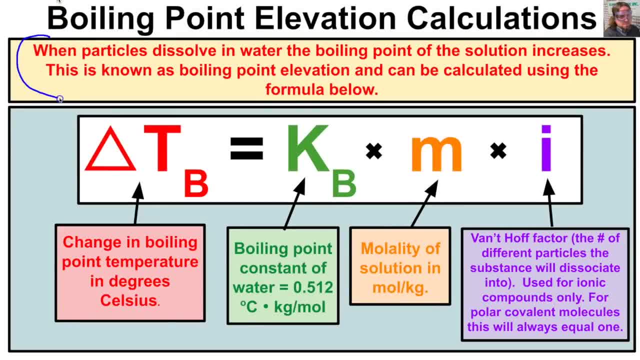 And so it says right here that when particles dissolve in water, the boiling point of the solution increases, And it says that this is known as boiling point elevation and can be calculated using the formula below. So we have the formula right here that the change in temperature of the boiling point, in this case of water- 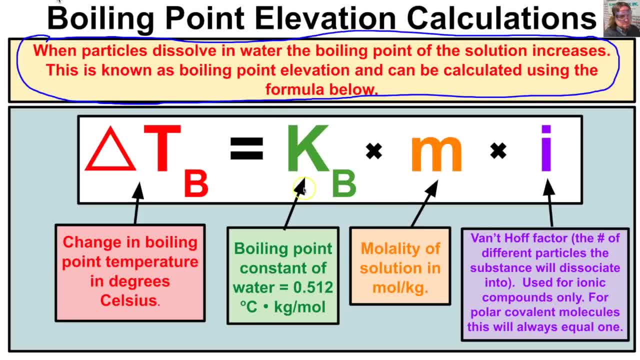 if we're talking about that, as the universal solvent is going to equal this right here: Kb, which is the boiling point constant of water, which is always equal to this right here: 0.512 degrees Celsius kilograms per mole multiplied by the molality of the solution. 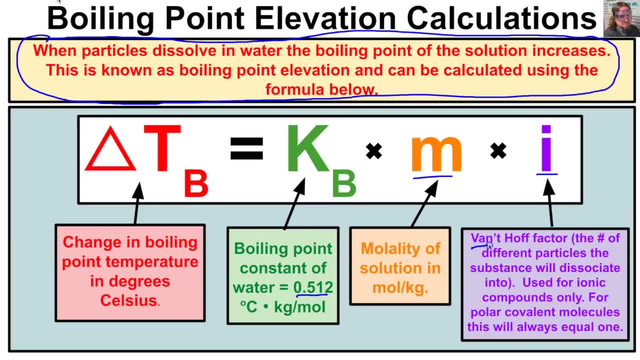 multiplied by I. What is I here? This is known as the van't-ha factor, And what this is is. this represents the number of particles that the substance or solute will dissociate into, And for polar molecules, this is always going to be a one, since it doesn't dissociate. 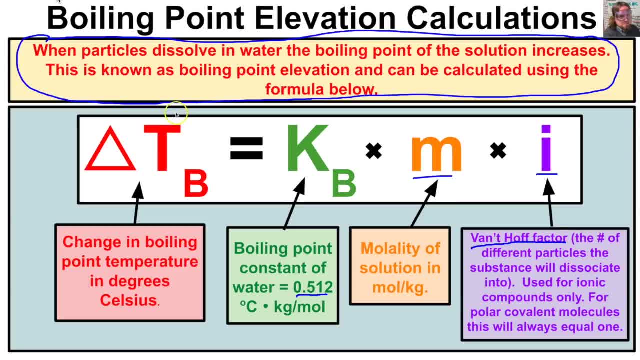 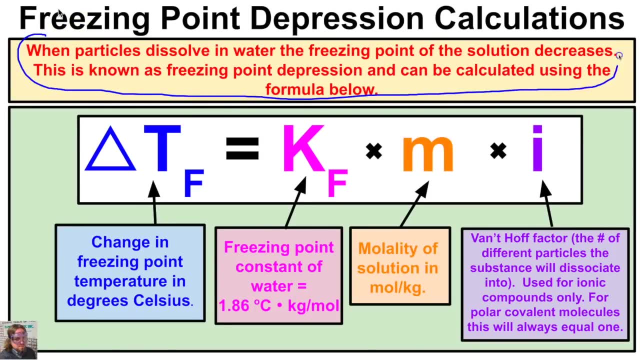 So let's take a look now at the freezing point depression formula and how we can use that to solve problems with dissolved particles in a solution. And so it says right here that when particles dissolve in water, the freezing point of the solution decreases, And this is known as the freezing point depression and can be calculated. 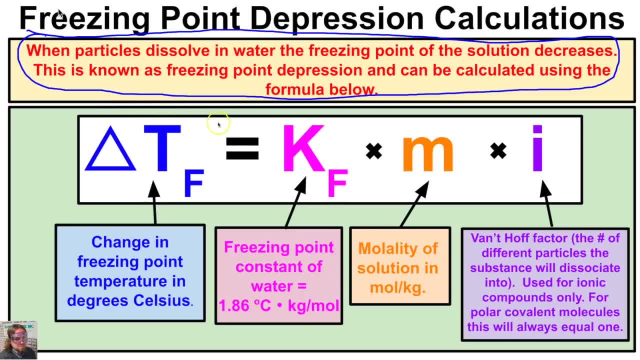 using the formula below. So the formula that we just looked at looks very similar to this, except it's for the boiling point elevation of different solutions, And this here is how we are going to calculate the freezing point depression of different solutions. And so, if we take a look, 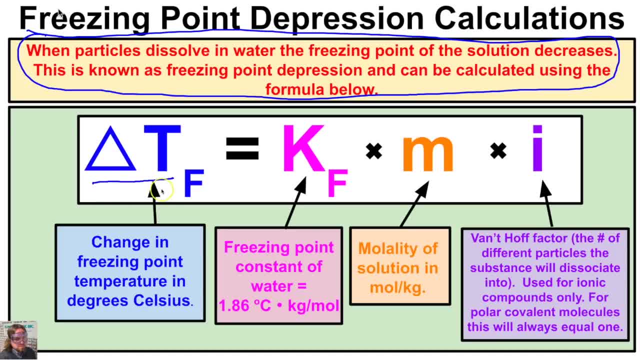 right here: 0.512 degrees Celsius kilograms per mole multiplied by the molality of the solution. 0.512 degrees Celsius kilograms per mole multiplied by the molality of the solution. we simply take the freezing point constant of water if we're talking about water as our solvent. 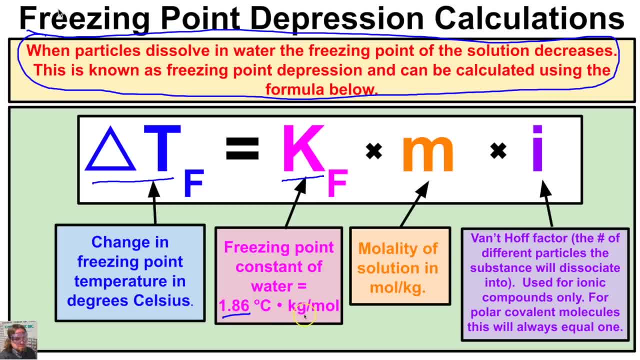 and that is going to be equal to 1.86 degrees Celsius kilograms per mole times the molality of the solution, times the van hot factor again. And so what we're going to do now is we're going to apply these two formulas to four different problems and hopefully you catch on. 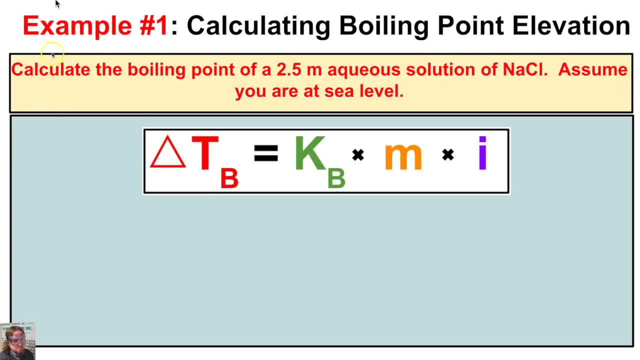 In this first example it says to calculate the boiling point of a 2.5 molal aqueous solution of sodium chloride. And we're going to assume we're at sea level And so we know that the boiling point of water at sea level is going to be equal to 100 degrees Celsius. So we know its boiling point at sea level. 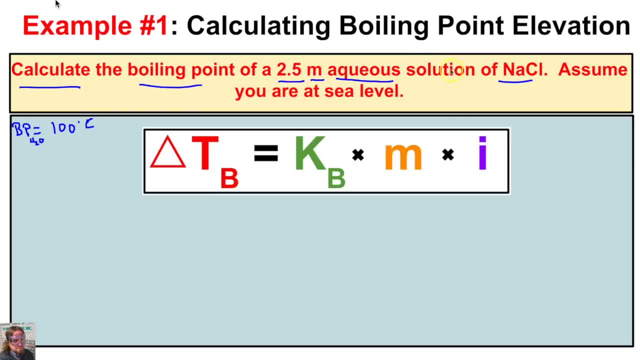 is a hundred degrees Celsius, And what we're going to do is we're going to add salt to this, to this water here, And so there's going to be a boiling point elevation. And so how do we calculate? 0.512 degrees Celsius kilograms per mole multiplied by the molality of the solution times, the van hot factor again. 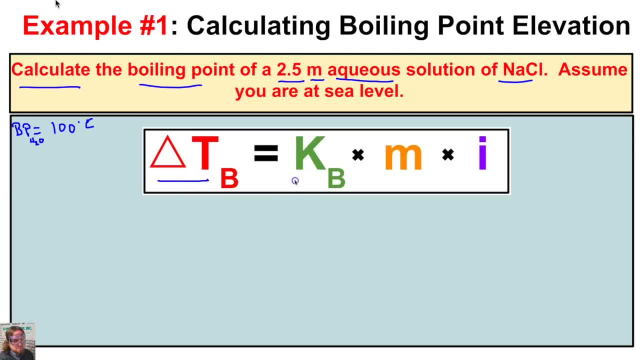 Well, to get the change in the boiling point, we take the boiling point constant times, the molality times, this I here, which is known as the van hot factor, And this here is essentially the number of particles that this will dissociate into when we put it in solution. And so if we 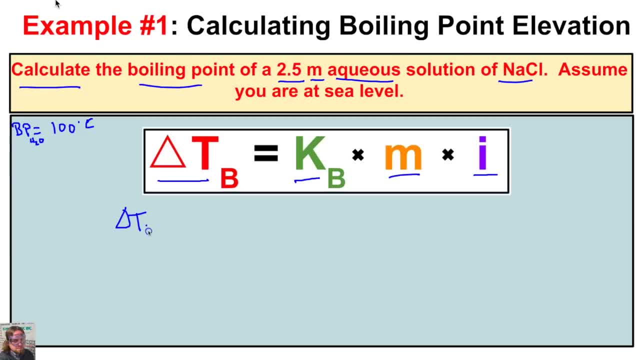 take a look here. let's go ahead and set this up to get the change in the boiling point of our solution. Now we're going to take the boiling point: constant times, the molality of the solution times, this thing called the van hot factor. And so right here, Kb, that is the boiling point. constant of. 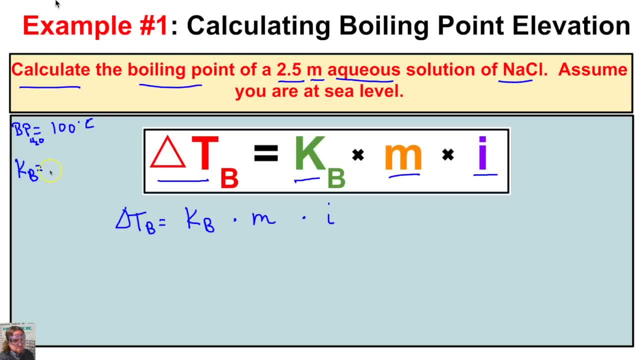 water, And this is different for every substance or every solvent. And if we take a look, the boiling point constant of water is going to be 0.512 degrees Celsius kilograms per mole, And so this was two. this was in a. we just talked about this when we talked about the boiling point elevation. 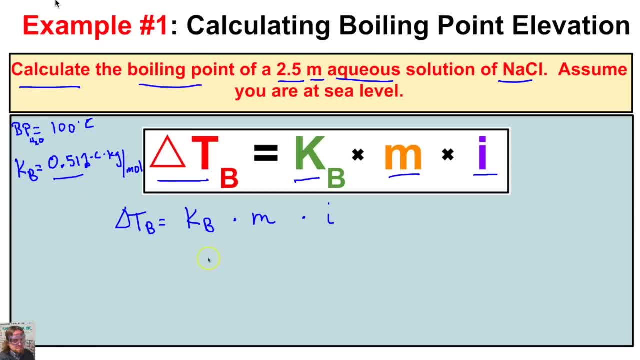 a couple of minutes ago. So this is a constant. This is always the same for water, So we'll go ahead and plug that in here: 0.512 degrees Celsius times kilograms per mole times the molality of our solution. This little M here stands for the molality of the solution And 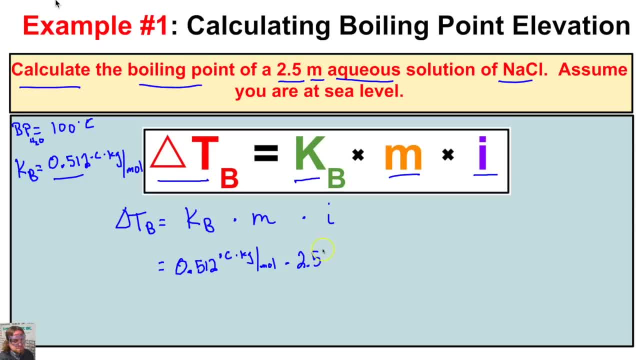 that is usually, or that is always, measured, when we're talking about molality, in moles per kilogram, And then we're going to multiply this by the van hot factor. And so let's think about this: If I have a beaker, if we have a beaker of water here, and we put this into water, if we take sodium, 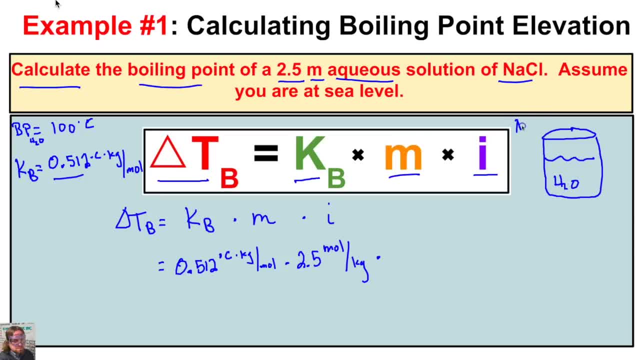 chloride and we put it in water. we know from an earlier video that this is going to dissociate. It's going to break apart into two different types of ions floating around in here: sodium ions and chloride ions. So this is going to break apart and dissociate into two, two different types of 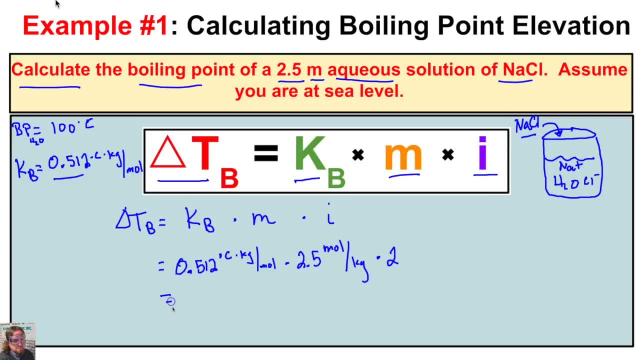 particles: 0.512 degrees Celsius, kilograms per mole times the molality of our solution. So this is going to break apart and dissociate into two two different types of particles. So our van hot factor here is two, And so now we just get a calculator out and we're going to take 0.512. 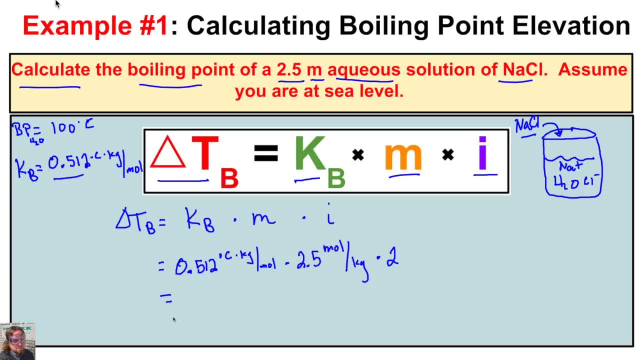 times 2.5 times two, And we're going to end up with 2.56, 2.56 degrees Celsius. If you take a look, kilograms is going to cancel out, moles is going to cancel out, leaving us with degrees Celsius. However, this is just the change in the temperature. This is. 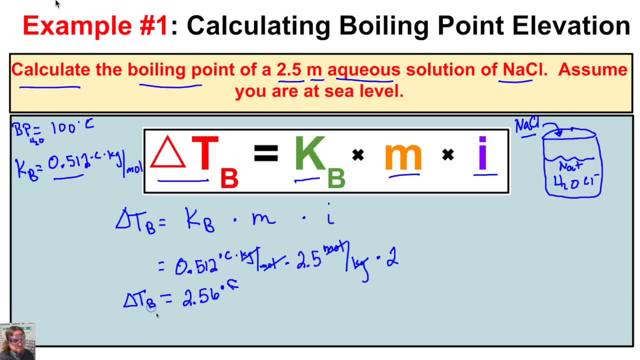 delta t. what we now have to do to get the boiling point is we have to take this and add this to our boiling point at sea level, and so we know that the boiling point of water is normally 100 degrees celsius at sea level, but we're going to add 2.56, since there's an elevation in the boiling point. 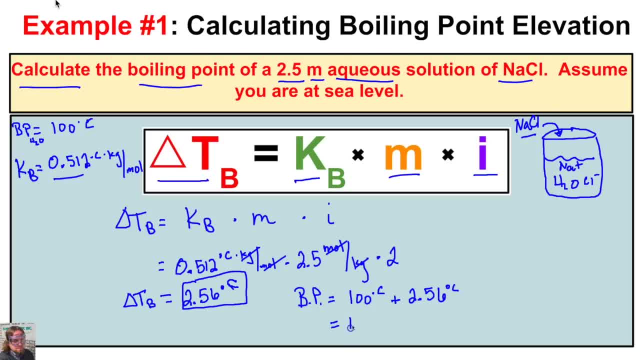 and when we put this in our calculator we should end up with 102.6. we'll just call it 102.6 if we're rounding to the 10th place degrees celsius. so when we add this salt to water it's going to raise its. 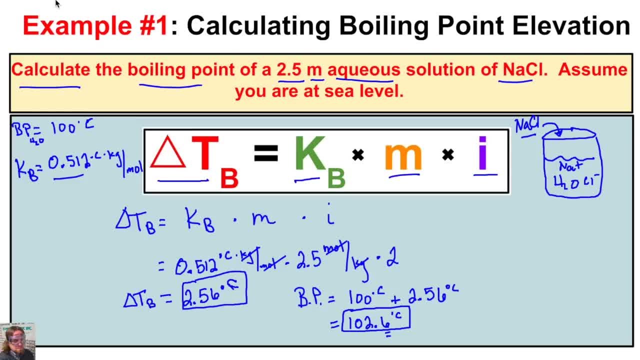 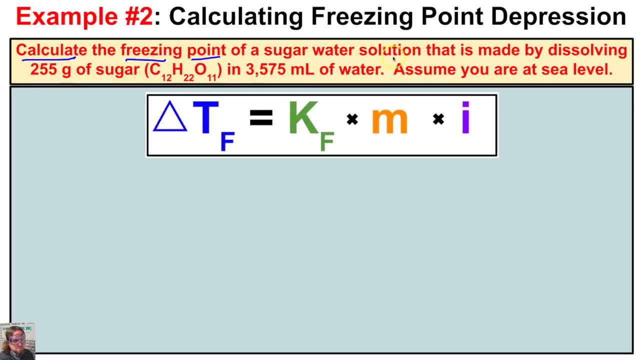 boiling point to 102.6 degrees celsius. let's take a look at another example. in this example right here it says to calculate the freezing point of sugar water solution that is made by dissolving 250 degrees celsius in water, and we're going to add this to our boiling point at sea level and 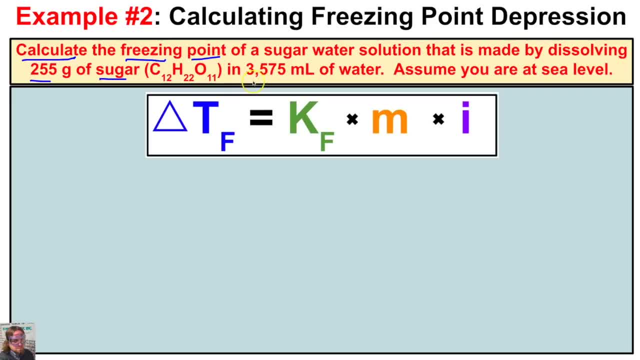 we're going to add 250 grams of sugar c12h22011 and 3575 milliliters of water, and we're going to assume that we're at sea level again, so the pressure doesn't come into play. and so, if we take a look here, we're dealing with sugar water solution, and so we're asked to calculate the. 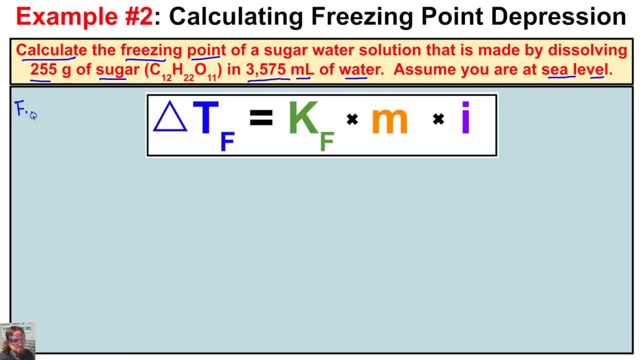 freezing point, and so normally we know that the freezing point of water is zero degrees celsius at sea level, and so what we're asked to figure out is the change in the freezing point, and so to figure out the change in the freezing point, and so to figure out the change in the freezing point. 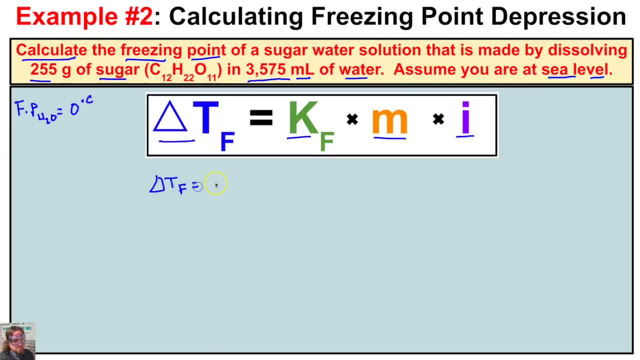 we have to take the freezing point constant of water times, the molality of our sugar, water times, the van't hoff factor, and so if we take a look here, let's go ahead and solve this problem. we know from a couple of minutes ago, when we talked about this formula right here, that 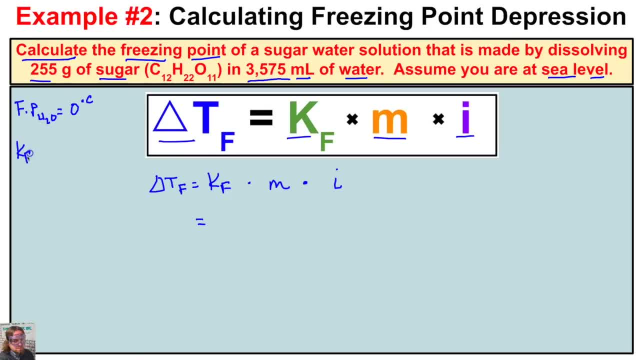 the freezing point constant of water is equal to 1.86 degrees celsius times kilograms per mole. so we're going to plug that in here: 1.86 right degrees celsius times kilograms per mole, times the molality of our solution. and so molality. what is molality? well, 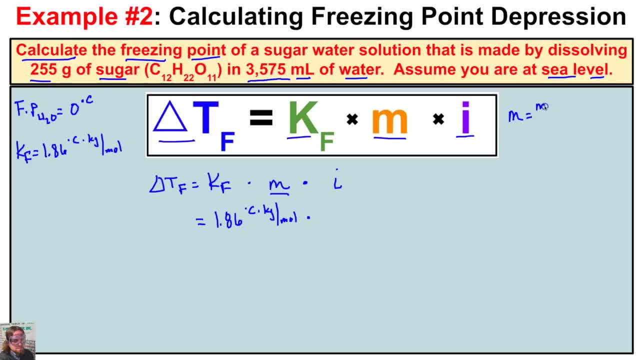 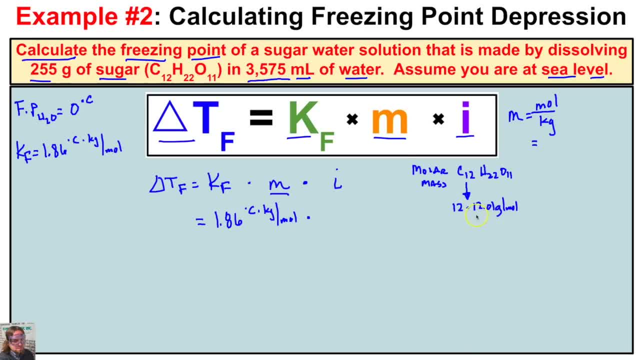 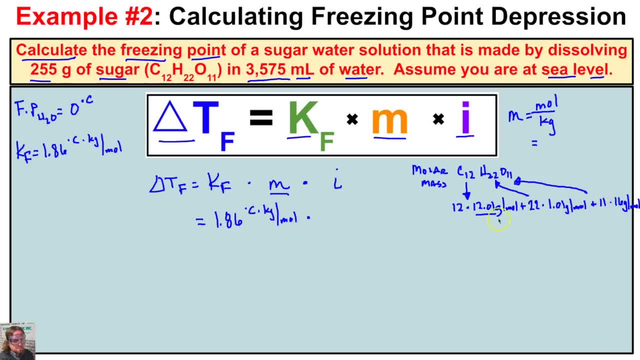 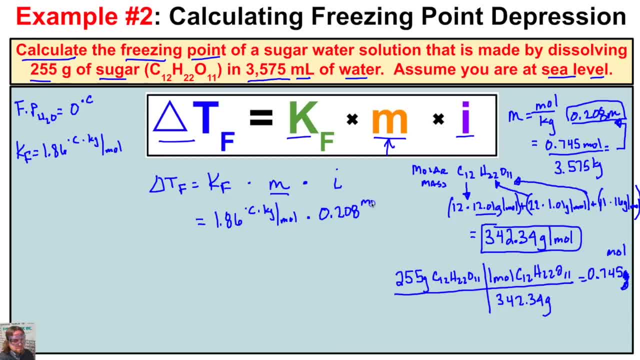 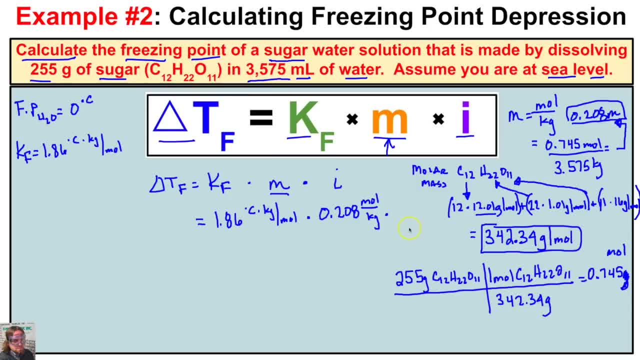 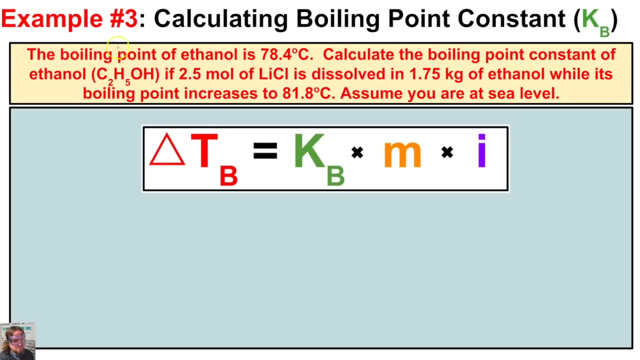 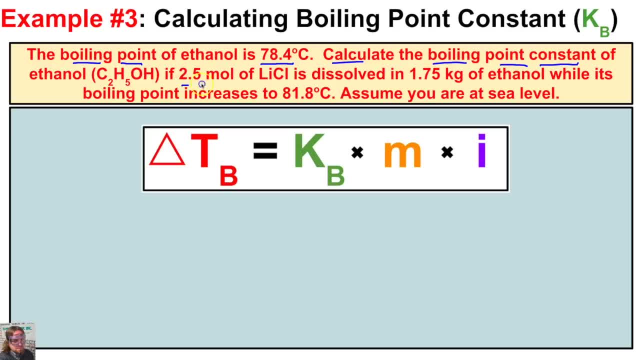 AB or the boiling point constant of ethanol. If 2.5 moles of lithium chloride is dissolved in 175 kilograms of ethanol while its boiling point increases to this right here, we're going to assume that we're at sea level. So there's a lot going on here. First of all, it tells us that the 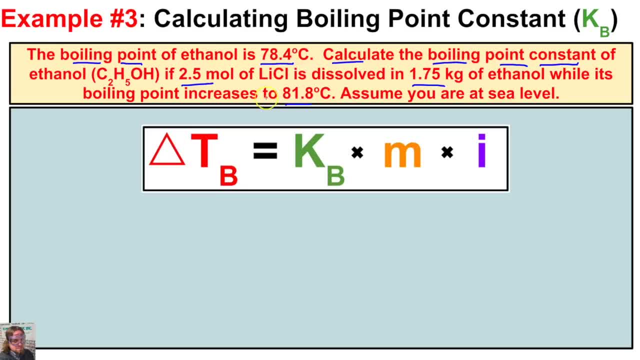 boiling point of ethanol is 78.4 degrees, We're going to dissolve some lithium chloride in it, And so if we dissolve lithium chloride in ethanol, it's going to increase its boiling point, And it looks like it's increased the boiling point to 81.8.. And what we're asked to figure out is the 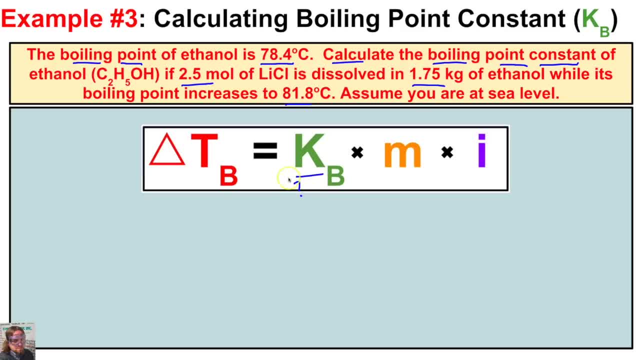 boiling point constant. We're asked to figure out the boiling point constant of this ethanol, And so what we could do is we could start to move this formula around. So if we know- we'll start over here- that the change in the boiling point temperature is equal to the boiling point, 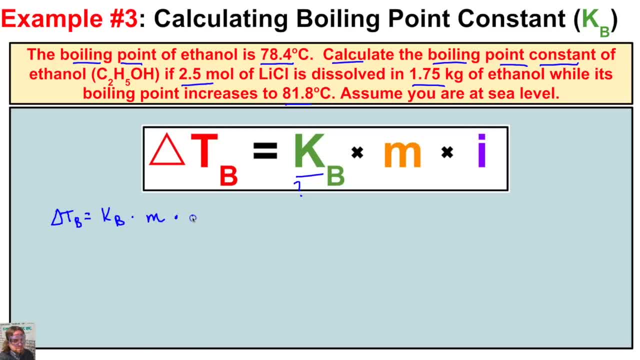 constant times the molality of the solution, times this van hop factor here, And we're asked to solve for this right Here. then what we can do is divide both sides by the molality, and I here will divide both sides by the molality, and I here or the van hop factor, And they're going to cancel from here. And so it looks. 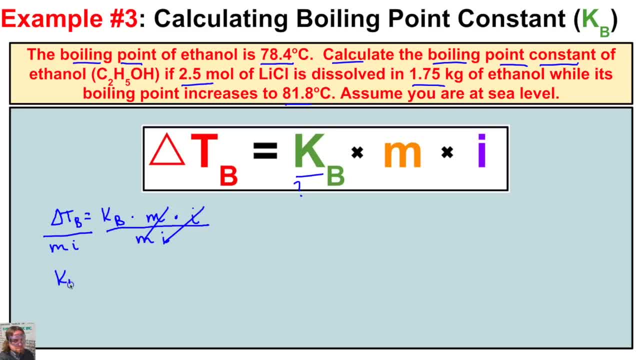 like to get the boiling point constant of our solvent, in this case ethanol. we take the change in temperature of the boiling point, or the change in the boiling point temperature, and we're dividing it by the molality, And so we're going to get the boiling point constant of the solution. 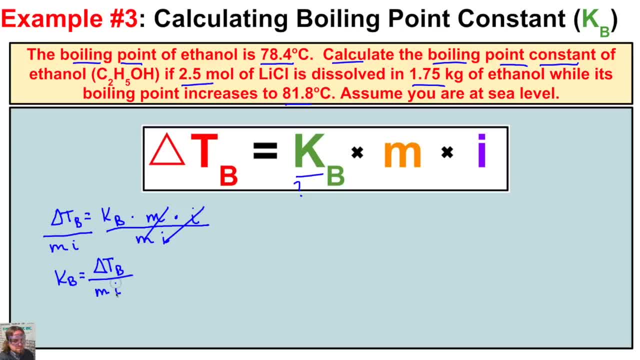 we're going to divide this by the molality times, the van't hop factor. so that's how we're going to solve this problem. so let's take a look further here. let's see here. we see first of all that the temperature, the boiling point temperature, starts normally at this right here it's 78.4 and it goes. 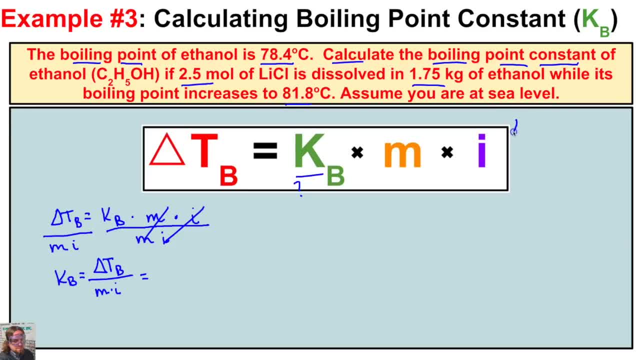 up to the right here. so how do we get the change in temperature? to get the change in the boiling point temperature, we take the final temperature minus the initial temperature, and so our final temperature is 81.8 degrees celsius. our initial temperature is 78.4 degrees celsius. 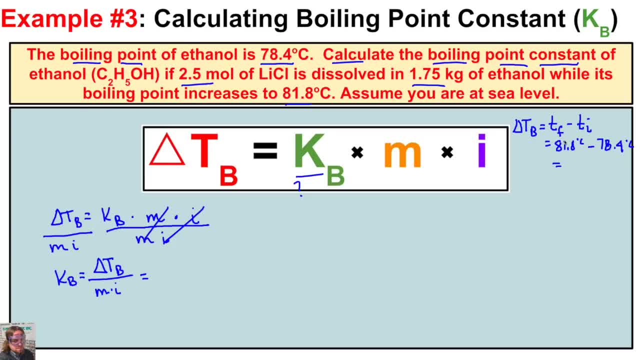 and when we put this in our calculator, when we take 81.8 minus 78.4, we're going to end up with 3.4. it looks like 3.4, so the change in temperature here is 3.4 degrees celsius, so we'll put that right here: 3.4. 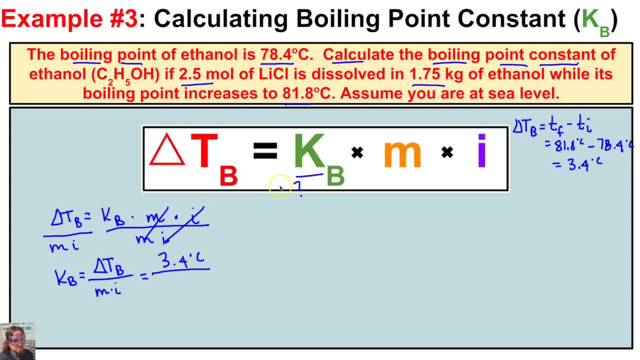 degrees celsius and we're going to divide this by the molality of the solution. now keep in mind that molality is equal to. molality is equal to moles of solute over kilograms of solvent. so if we take a look here, what are we dealing with? we have 2.5. 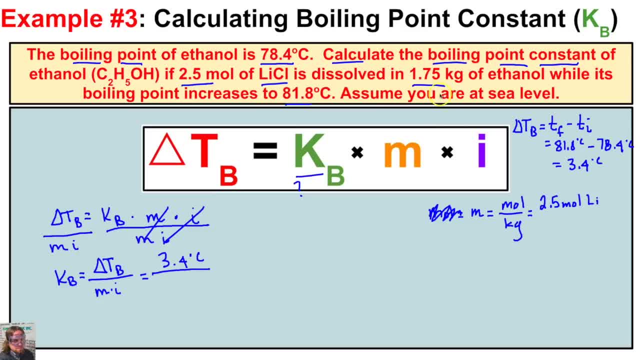 moles of lithium dissolved- it says right here- in 1.75 kilograms of ethanol, which is our solvent. so we have 1.75 kilograms. so when we put this in our calculator, 2.5 divided by 1.75, we end up with 1.43, approximately 1.43 as the molality of our solution. 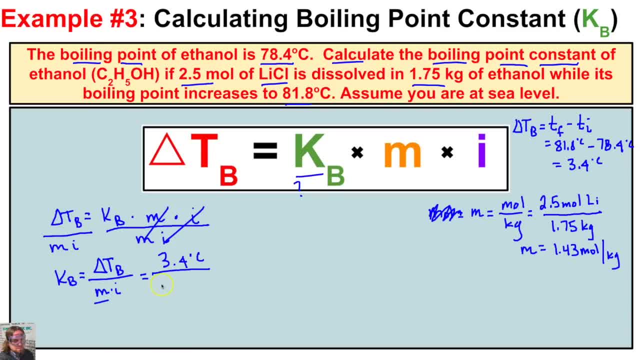 so we'll go ahead and put that right here. we'll substitute that in 1.43 moles per kilogram, so that's what you're looking at. so we pick up the rate at 12.. Outside the fourth fig, να cäl our solution right here. so our van hop factor is going to be 2, so we'll put. 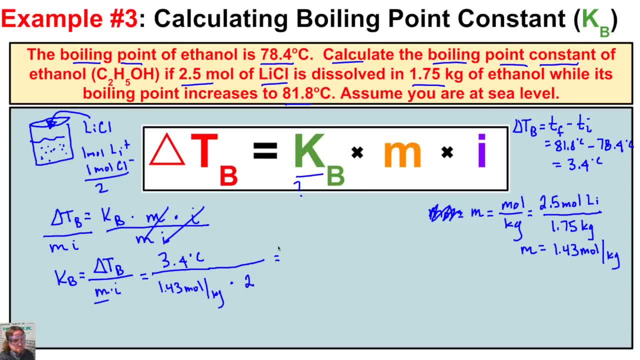 this in our calculator: we take 3.4 and we're going to divide this by and if we put in the denominator here, if we multiply these to you to two terms, we need to put them in parentheses in our calculator- 1.43 times 2 and we're going. 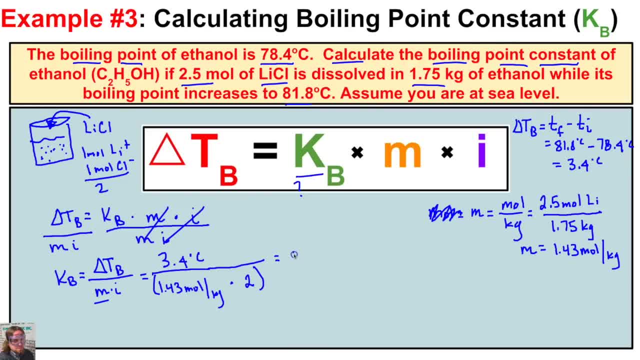 to end up with one point one nine, approximately one point one nine. what well, if we take a look, our units left over are going to be degrees Celsius, and if we flip this to kilograms per mole, then we multiply by it, not divide by it. so we're gonna hit. we're gonna put times kilograms per mole. so there is our. 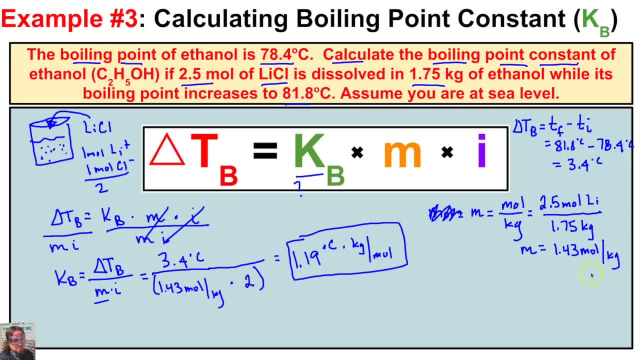 boiling point constant of ethanol. so if you like this video and you like what you see, go ahead and click that little bomb in the bottom right hand corner and that will subscribe you to my channel. and feel free to leave any comments or questions in the comment section down below, and I really hope you guys found this helpful.